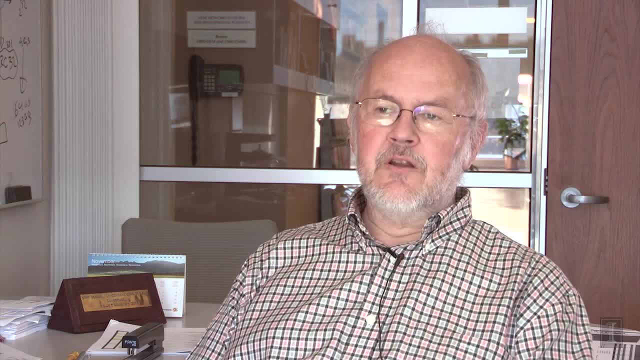 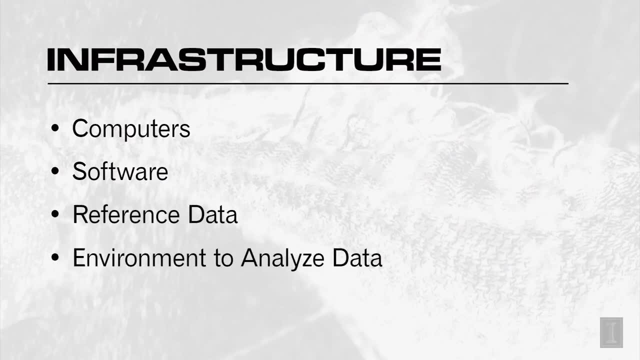 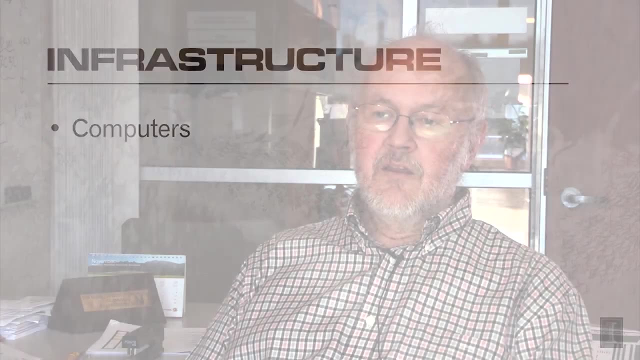 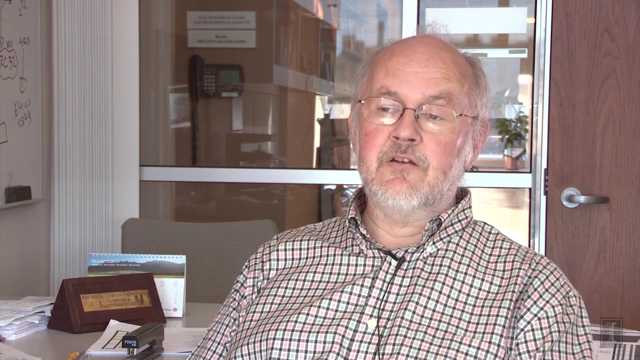 missions. The first one is to provide infrastructure, And infrastructure means computers, software, reference data, an environment that people can use to analyze biological, biomedical data. By the way, this infrastructure also supports the high throughput DNA sequencing center at the Biotechnology Center. 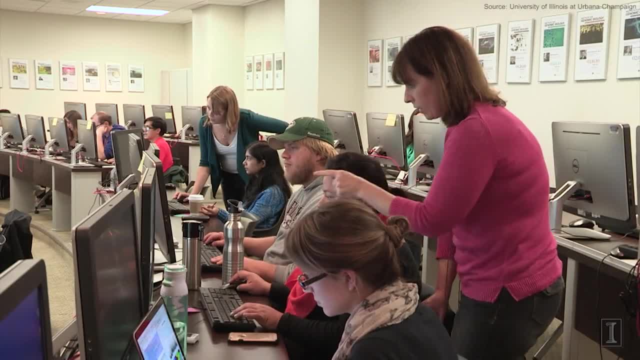 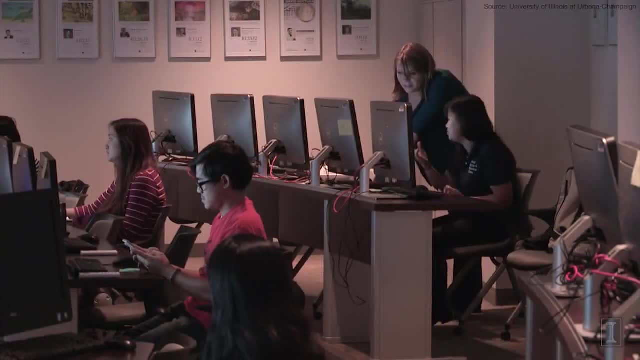 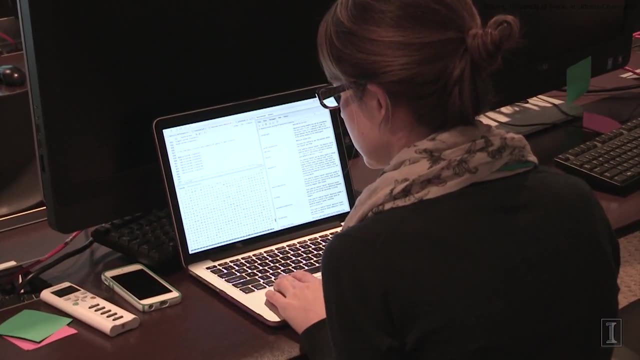 to be on campus. We want everybody to be on campus. We want everybody to be on campus. We would like our biomedical researchers to be eternally dependent on us. We'd like them to be able to use the computational facilities to analyze their own data and require less. 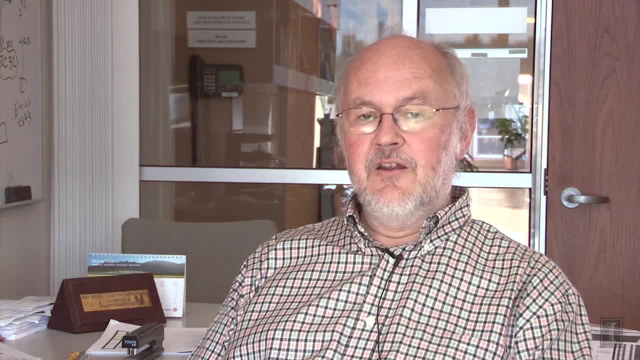 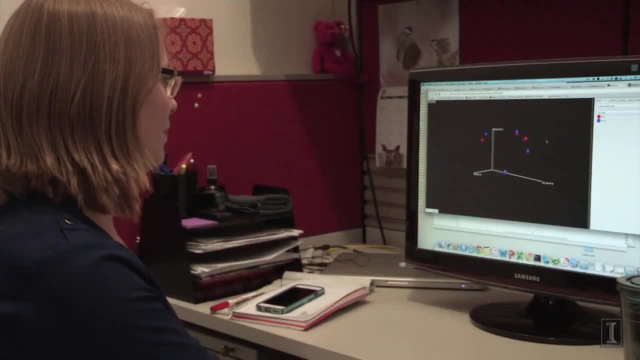 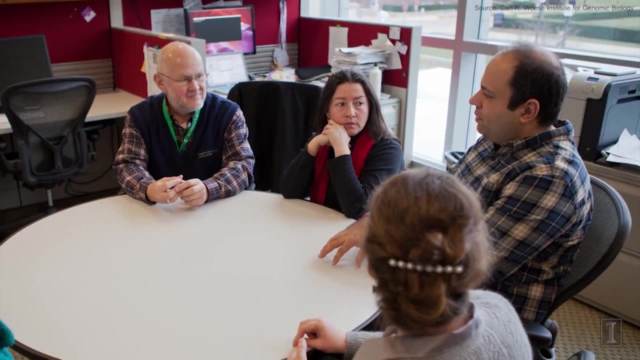 and less help from us. The third mission is support, and by support I mean providing an environment where campus researchers can come to us, ideally before they even do their experiments, where they're just thinking about it, and then they can come to campus and they can do their experiments. 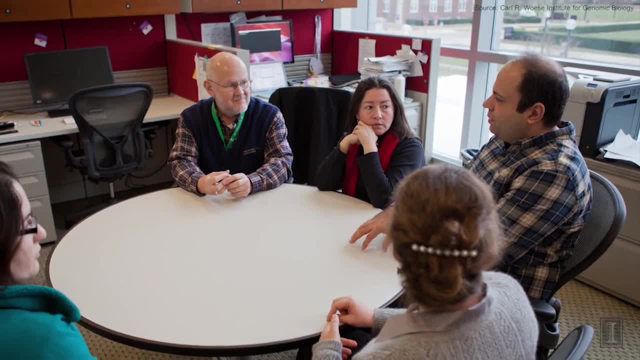 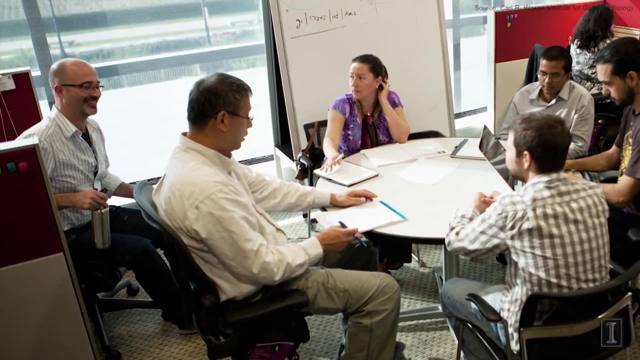 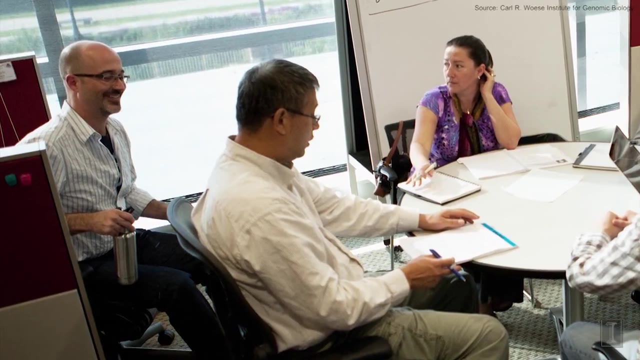 a project and they're thinking about how are we going to do this from a technical point of view, and we help them define how to best apply techniques, how to best gather their data, what technologies to use, and then afterwards, of course, the main part of the work is that we help them analyze the data and make sense out. 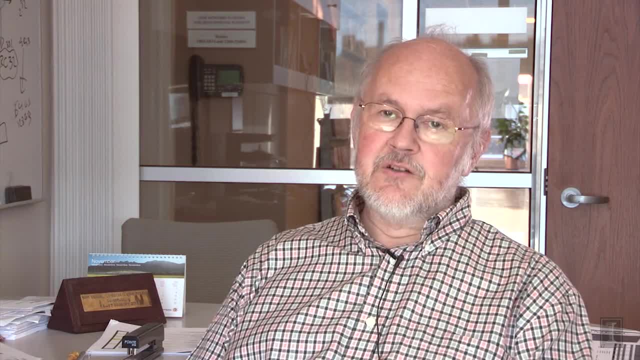 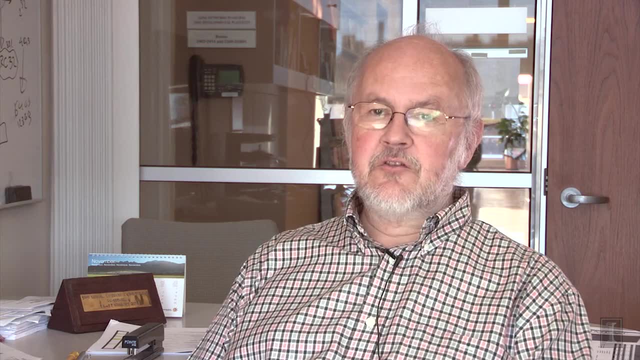 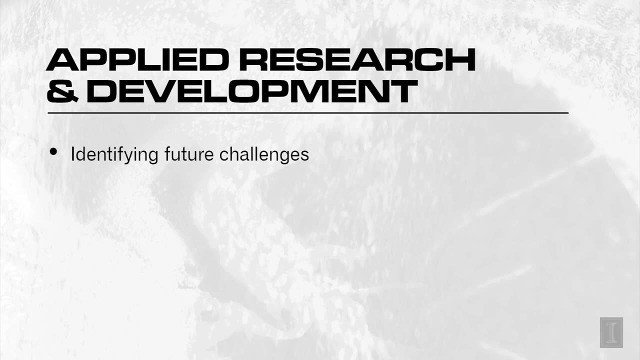 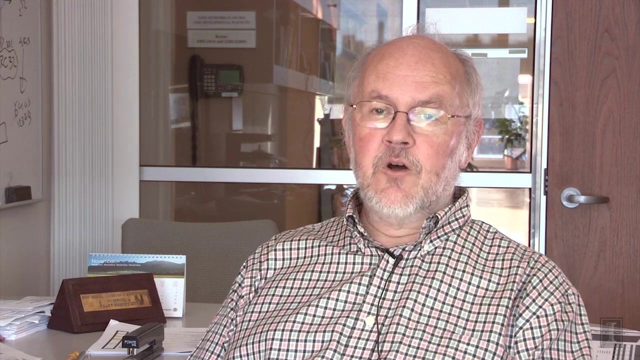 of it. the fourth mission is a little unusual for a service oriented facility, and that's to do what we call applied Rnd. and applied rnd means thinking about where our work is going to be going over the next few years and thinking about what kinds of things we will need to be able to do and prepare for that. and 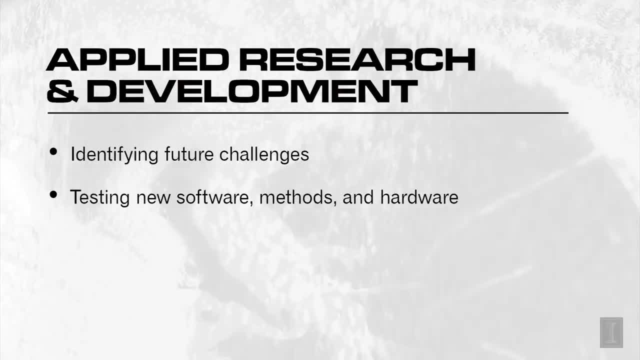 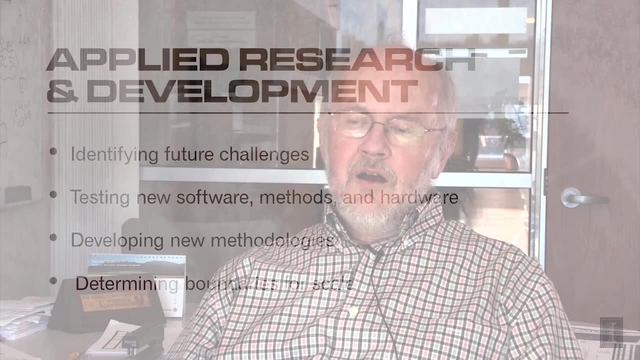 that's the end of my presentation. That means sometimes testing new software, new methods, testing new hardware, sometimes developing methods, sometimes exploring the boundaries, in terms of scale of what we are able to do. So all of these activities that kind of prepare the future. 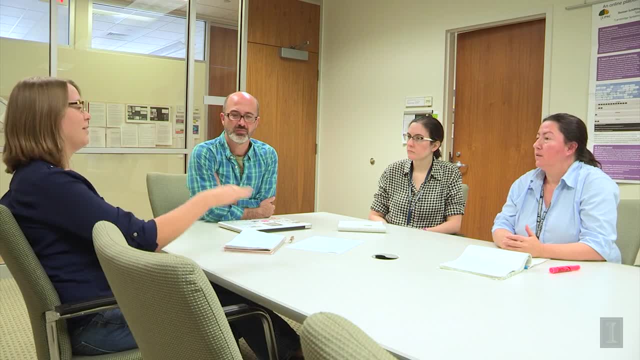 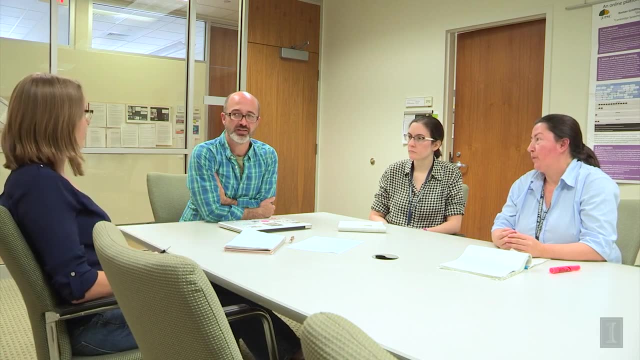 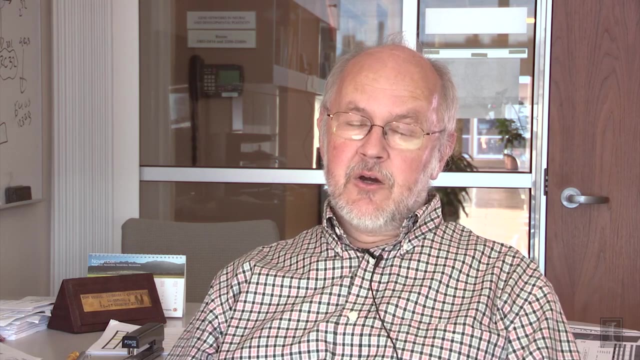 We have a staff of about a dozen people now, So we have part of our staff- are the people who interact primarily with the biologists and who help them define their problems and solve them, And these are all people who had basic training in biology and then followed up by getting 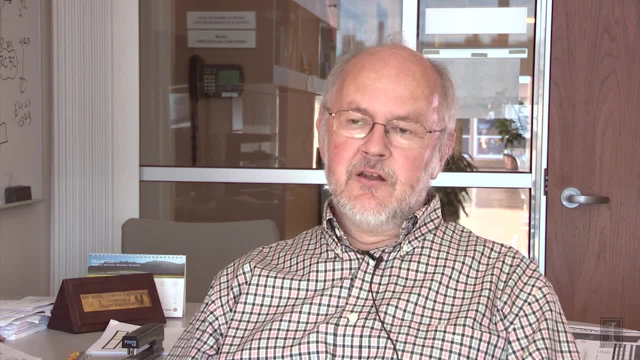 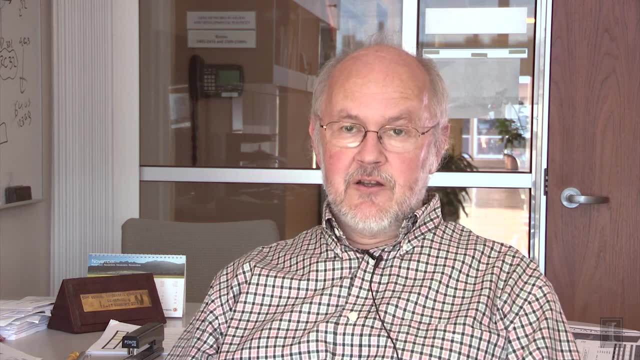 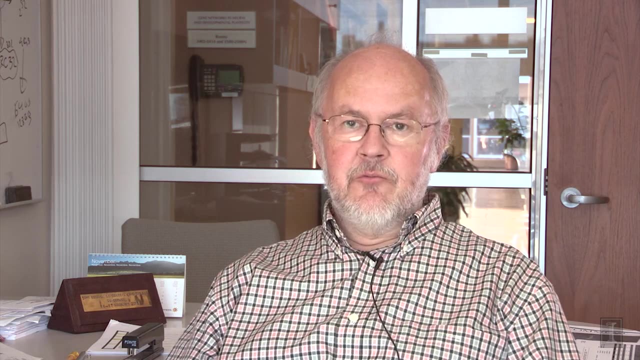 also some amount of training in computational science. On the other side, we have a group of people who are primarily computational scientists and who really know how to put together the machines, how to make them work and so forth, And who are very high quality programmers. 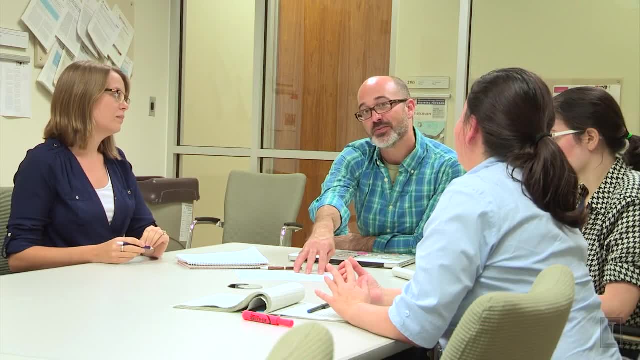 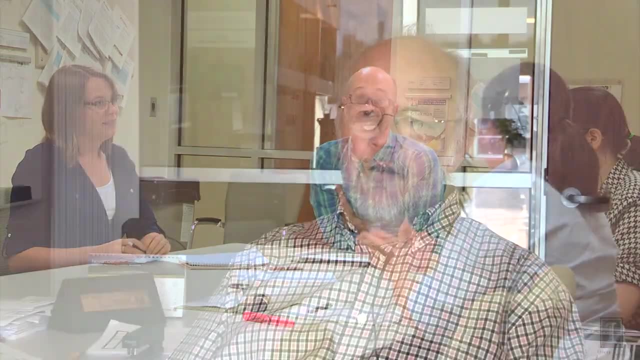 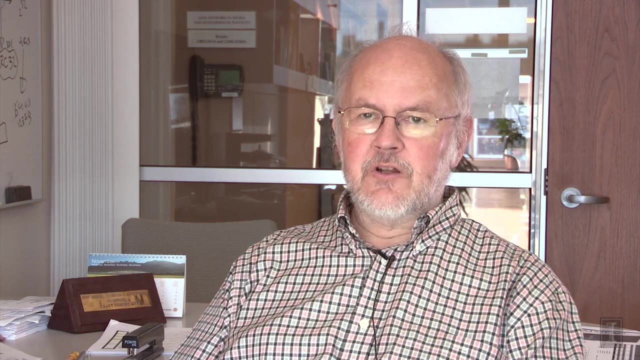 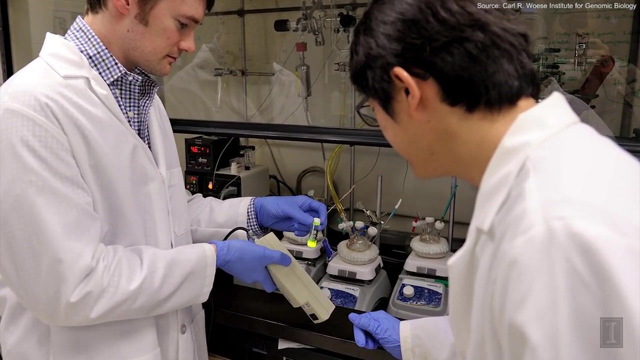 But these people have to work together on a regular basis and talk to each other all the time, And that is really how you put a team together. So we are a different university for most in the countries, in the sense that the research strengths on campus here are not. 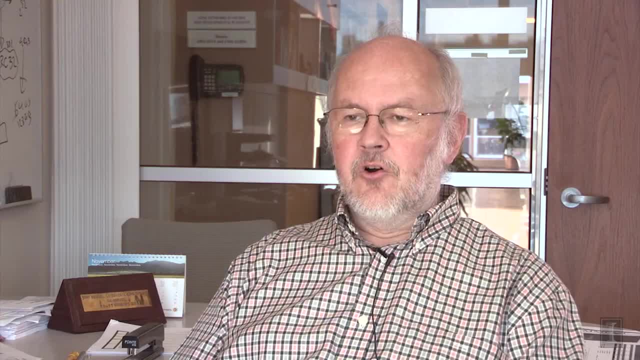 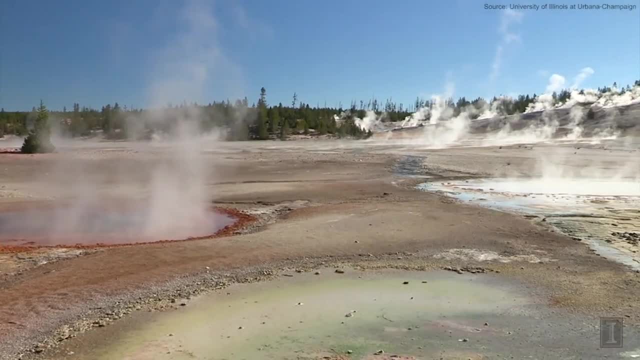 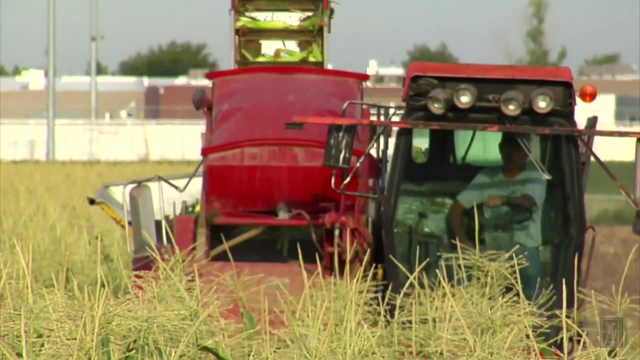 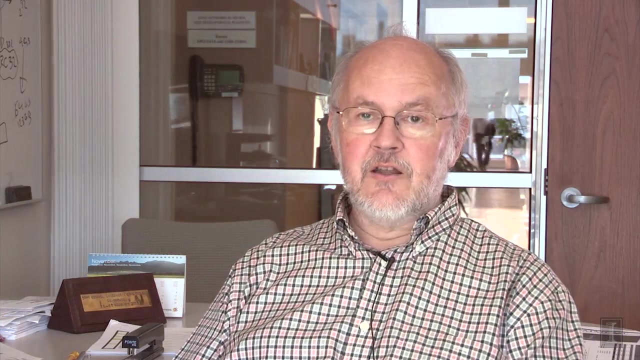 In kind of traditional biology and medicine. So there is a huge breadth of interest on campus in exploring life in all of its dimensions and in ways that it affects the environment. it affects agriculture, farm animals, crops, And because of that we have a much wider portfolio of projects than you would find. 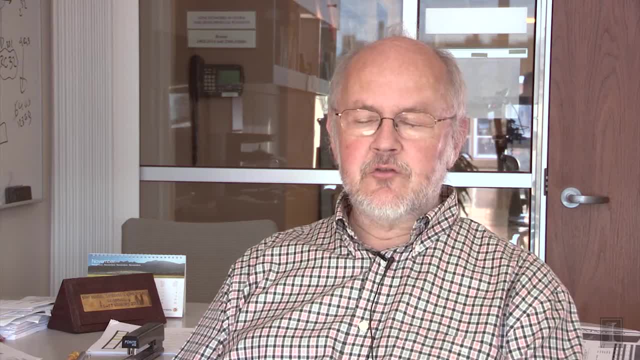 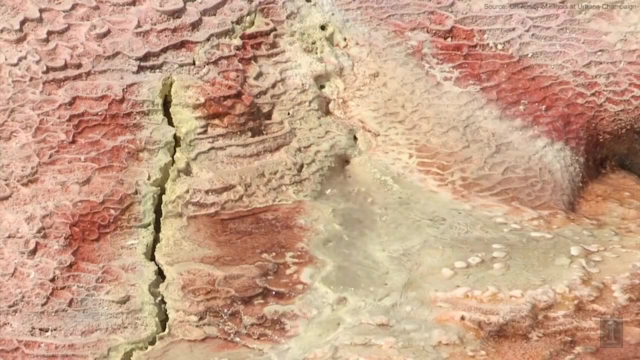 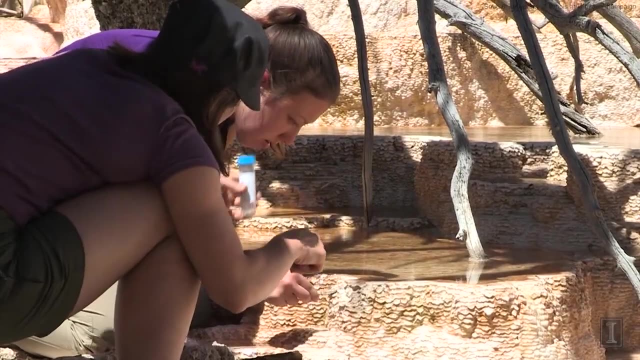 in most facilities that would be in our peer institutions. So that is really what we do. So, to give you an example, we have done a lot of work looking at bacterial and archeo communities that live in hot springs in Yellowstone Park. There are several faculty members on campus who are interested in that. 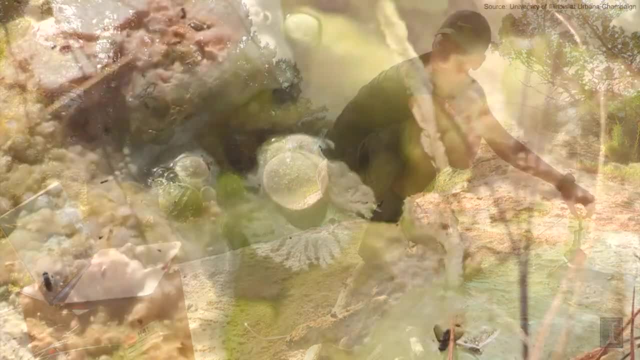 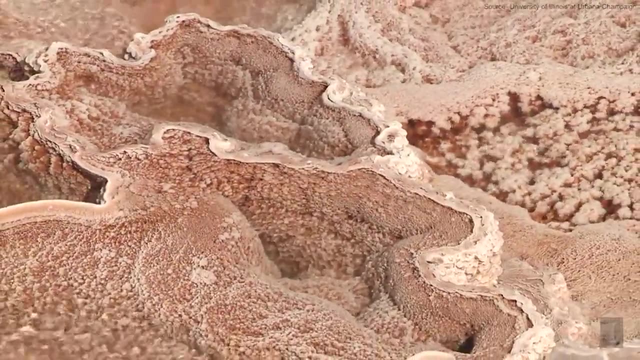 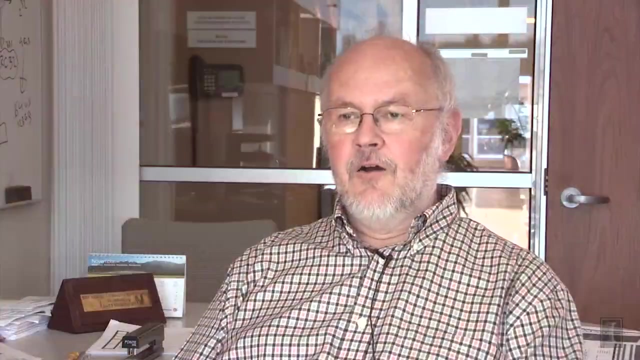 And by sequencing their collective genomes- what is known as a metagenome- we have learned a lot about how they live and what kind of things they metabolize and how they manage to survive in a very hostile environment. We have also had a number of projects on agricultural pests, where we look at their